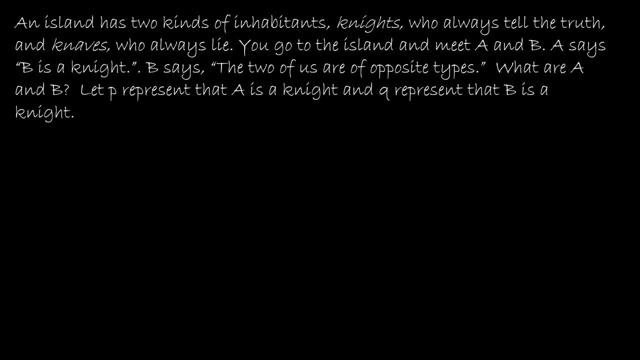 question. it says we go to the island and we meet A and B. So we've got person A and person B. A says B is a knight, B says the two of us are of opposite types. What are A and B? So we're going to let P represent A is a knight and we're going to let Q 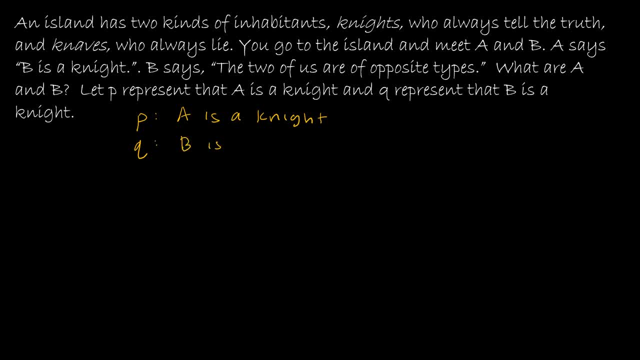 represent B is a knight. So there's a lot of different ways to go about this and again, there's no one correct way to go about this, but there is one correct answer. But to kind of get us started and to make sure that we're staying organized, we really have four possibilities. We either have P is Q. 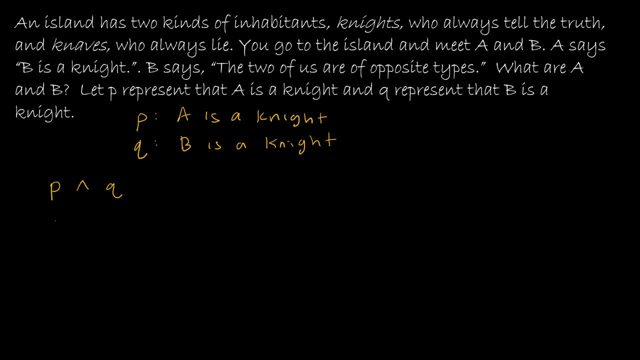 and Q is true. We have P is true and not Q. We have not P and Q, or we have not P and not Q. So here's my options. and again, we're thinking about this in terms of knights and knaves. So let's just reason through it and I'm going to show. 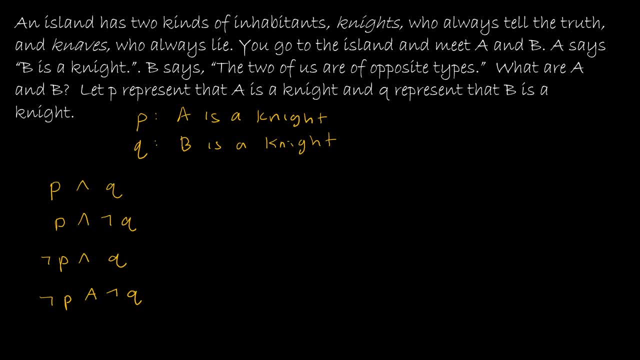 you an example in a second where we can do this with sort of a modified truth table. but let's just use our reasoning Here. we have that let's. let's start by assuming this is true. We go to the island, we meet A and B. A says B is a. 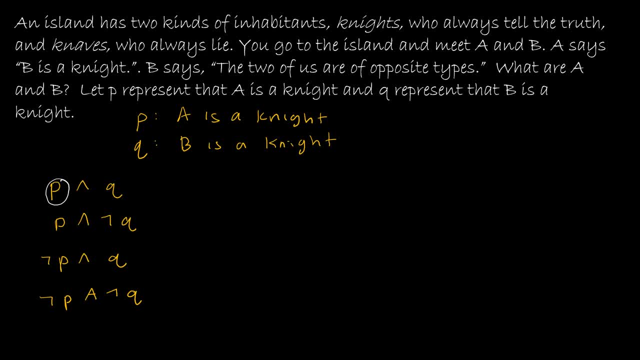 knight. So if A says B is a knight and we're saying P is true, so we're saying A is a knight And A says that B is a knight, Okay, so that works out okay for A's statement. B says the two of us are of opposite types, So are P and Q of. 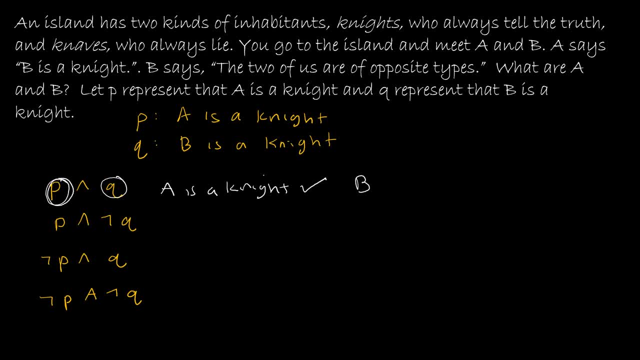 opposite types. No, because we're saying right now that A said that B is a knight. but if B is telling the truth and they're of opposite types, then this logically doesn't work, because B can't be a knight and be telling the truth about A and B being different, So doesn't work. This next one says A is a. 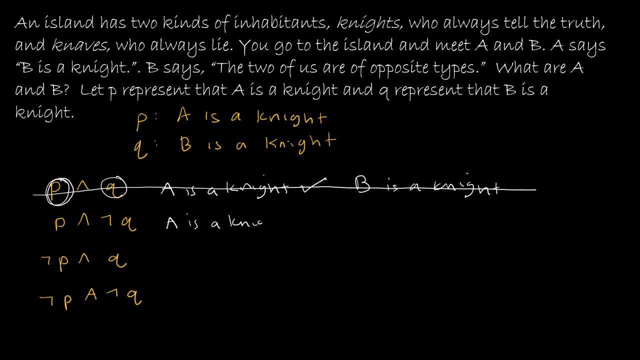 knight and not Q would say B is a knave. So our first statement says A is a knight, B is a knight, So A is a knight, and telling the truth and telling us that B is a knight. but we know from here. we're saying B is a knave, so this one doesn't. 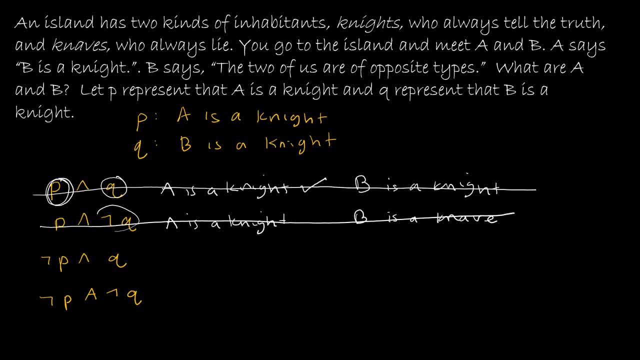 work. It's faulty logic. So we're down to two options. This one says A is a knave and therefore is lying right, and B is a knight. So let's see if this one could work. A says B is a knight, So A is a knave and says B is a knight, but A has to be lying. 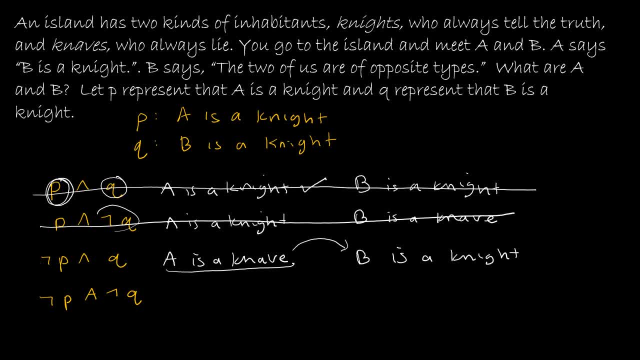 And if A is lying, then that means B must be a knave. So this one doesn't work. So clearly by elimination. this is our solution. but let's take a look. This one says A is a knave and therefore lies, and not. Q means B is not a knight or B is a. 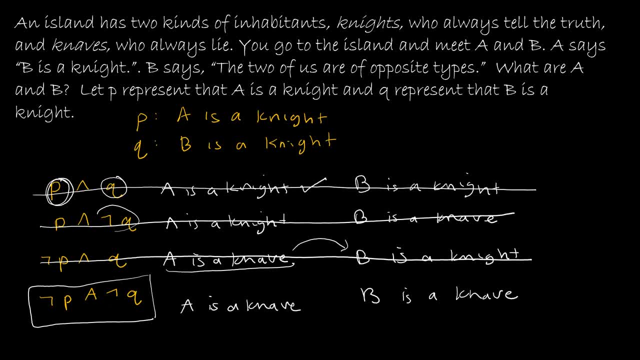 knave. And now let's make sure the logic holds. A says B is a knight, okay, and is lying, because he's a knave and lies and therefore his works out okay. B says the two of us are of opposite types, which would mean he would have to be a knight. 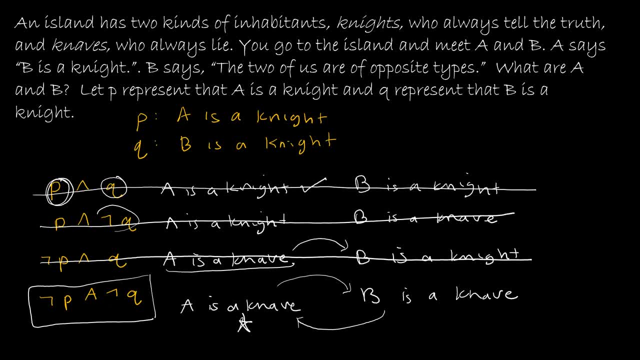 except that he's lying, and so that means he's saying there were the same type, So his statement holds true as well. So our only solution is that both A and B are knaves. Here's another way that we can go about solving this, and this is using: 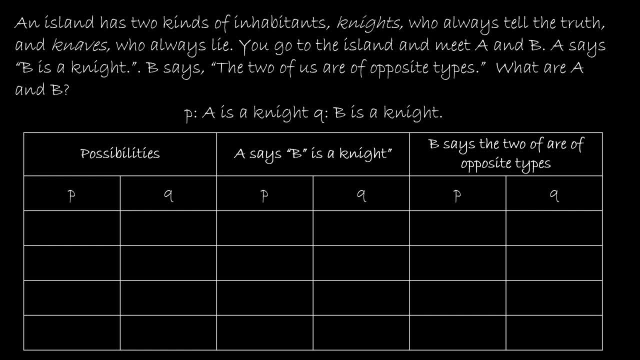 a truth table, And we should be familiar with truth tables to this point. but remember, on a truth table, the very far left side is just going to be our possibilities. So we're using P, that A is a knight, Q, that B is a knight, and so we. 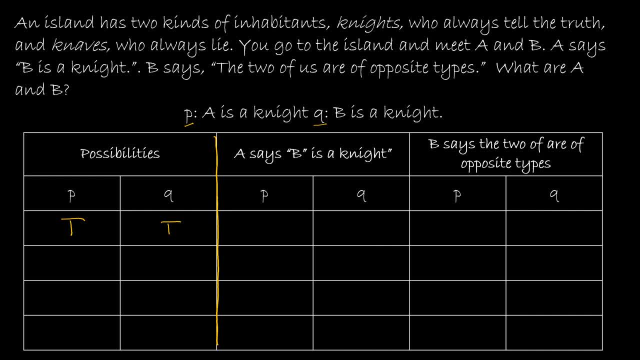 can have the possibilities of true, true, true, false, false, true, false, false. Those are all our possibilities Now when we're doing a truth table like this. essentially what I'm looking for is: I want whatever happens in this set of columns to match up whatever happens in this set of. 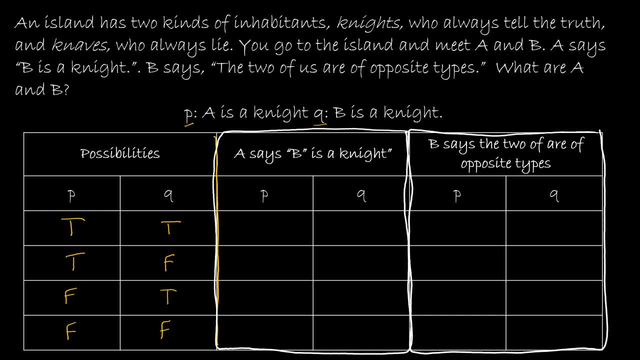 columns, And if that's the case, then they are equivalent and therefore everything's okay. So let's take a look at what I mean by that. Let's just start working through this together and hopefully, if there's any confusion, I can clear it up as we go. 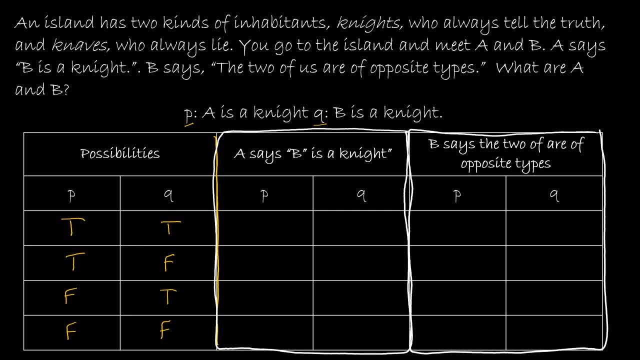 through. When I'm going through this for my first statement, I'm assuming that the P is exactly as P is in my combination. So I'm going to do true, true, false, false. and for B says two are of opposite types, I'm going to assume that Q is whatever, Q is over B. 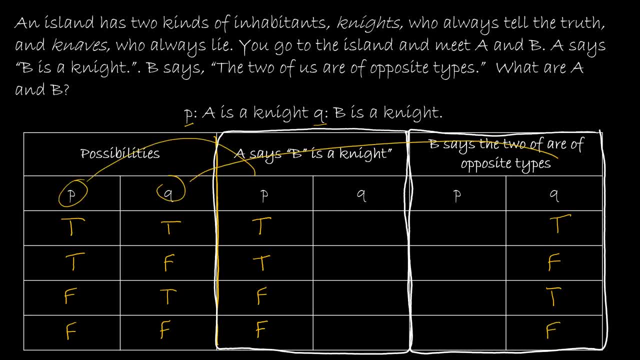 and so let's just start over here. So I've just recopied P and recopied Q and then I'm going to evaluate Q here based on P and I'm going to value that P here based on whatever Q says, And then hopefully we can find something where everything matches up and works out. 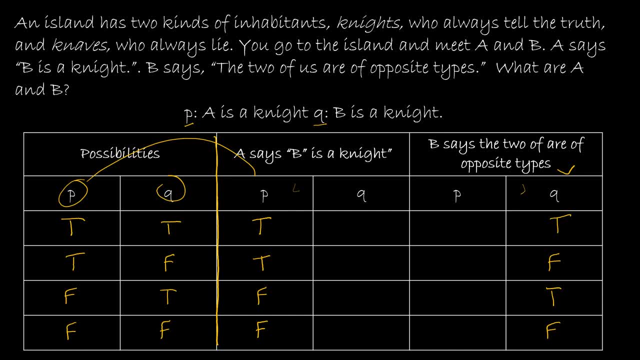 So let's get started. If A says B is a knight- And that's what we're saying here- that P is true, So P is a knight and A says that B is a knight. therefore B or A is telling the truth, and B must be a knight. 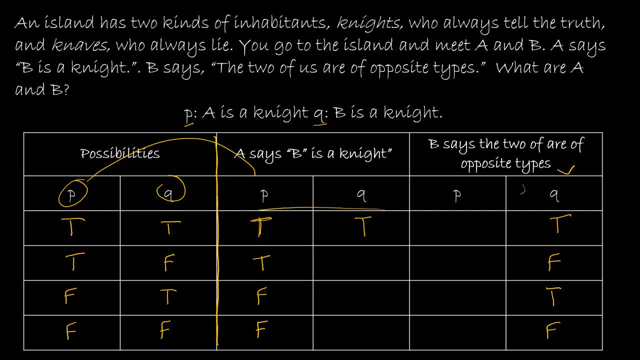 And therefore this one's okay, because we see true true, which matches with true true. So if we get a true here, then we know that we're correct. So let's take a look. B says the two are of opposite types. 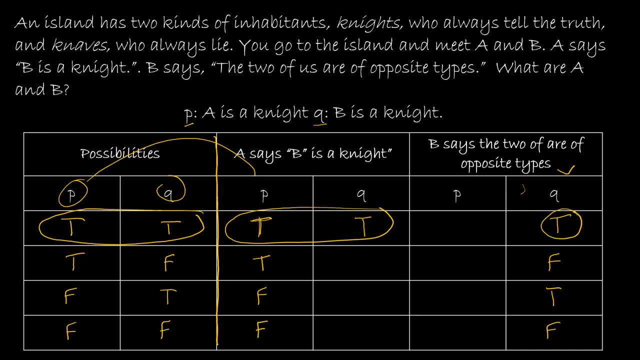 So if Q is true he's a knight, then the knight is saying the two are of opposite types, and that tells me that P must be a knave or that P is false. So notice, this does not match up and therefore this is not a possibility. 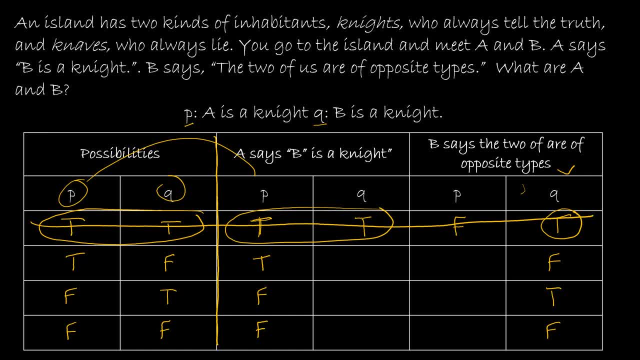 So let's continue that same method Again. I've already filled in the true for P, So I'm saying A says B is a knight, A is a knight, based on this statement right here and telling the truth, and therefore, 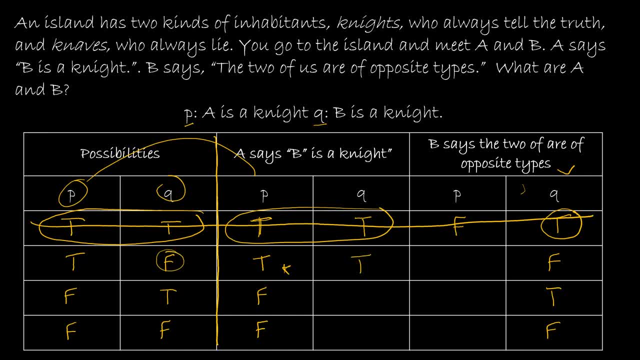 this must be true, But we know that it can't be true and therefore I'm not even going to check anymore, because that one is not going to work. Let's try again. I have false true. So A says B is a knight. 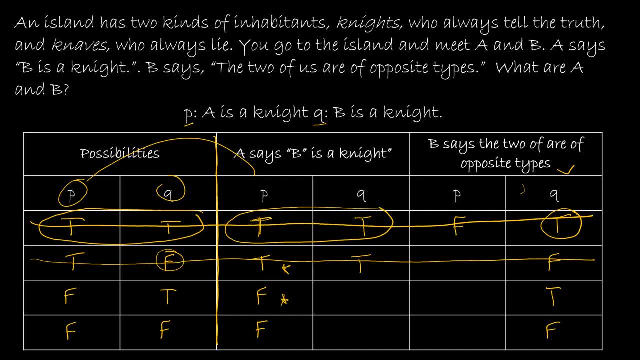 but A is a knave and therefore is lying. So if this one is false, then this one, because he's lying, must be false. And again, that doesn't match up and I don't have to continue. 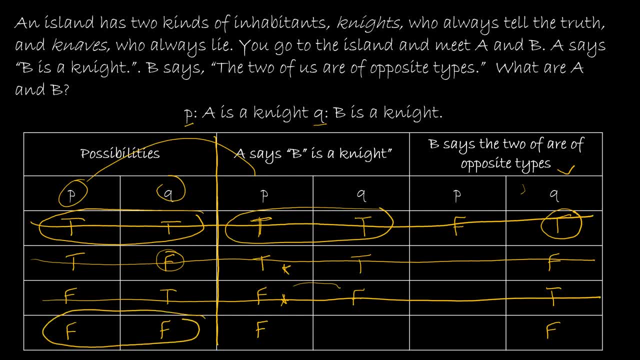 We already know that this is the answer, because we just did this question, but let's go ahead and check it. A says B is a knight, but A is a knave, and so he's telling a lie. therefore, it must be that Q is false. 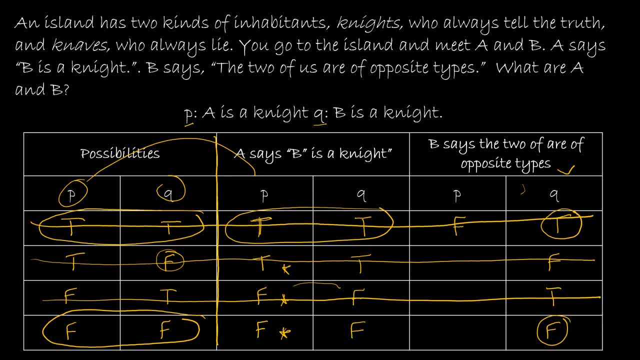 Let's try this one. We have B, says the two are of opposite types, but he's a knave and therefore lying, and so this must also be false. So notice, this is the one that matches up. So, just as we did it before, without a truth table. 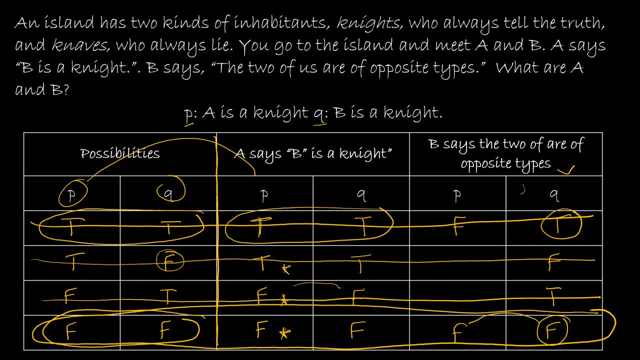 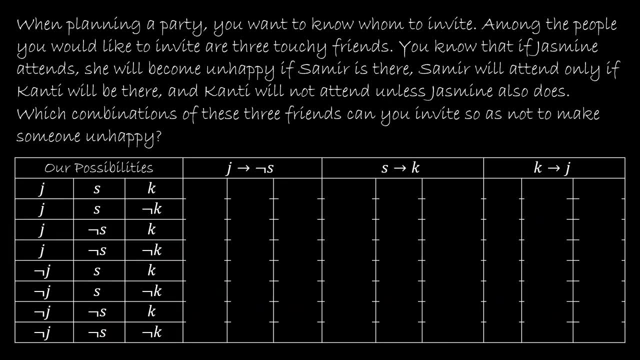 we came to the same conclusion. This is just a way for us to come up with the same solution using a truth table. So let's take a look at another logic puzzle. We are planning a party and we're going to have a party. 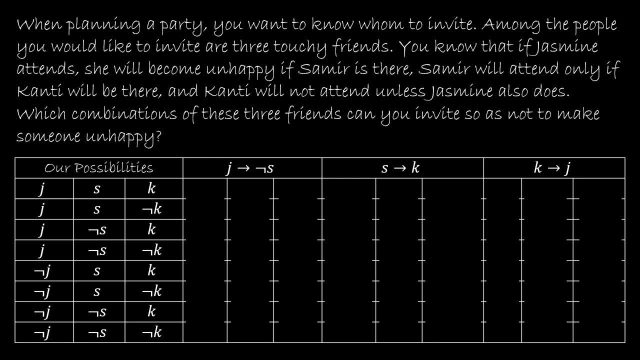 and we have some very sensitive, touchy friends who don't want to be there if other people are there, and so, as you can see, I've already started this truth table for you and I didn't use true-falses this time. 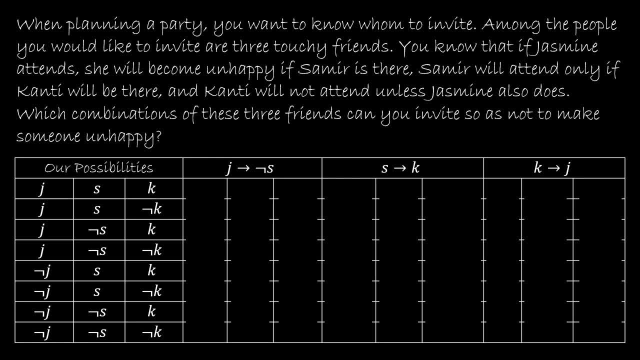 What I did was kind of like what I did on that last one, where I just did not Ps and not Qs, but I'm using J, S and K to represent Jasmine, Samir and Conti, our three very touchy friends. 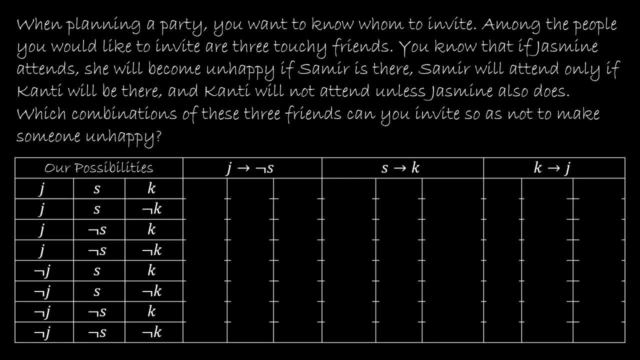 So the first thing I did was I looked at the sentences in the question, and this one says: if Jasmine attends, she will become unhappy if Samir is there. I translated that to be: if Jasmine is there, then that implies Samir was not there. 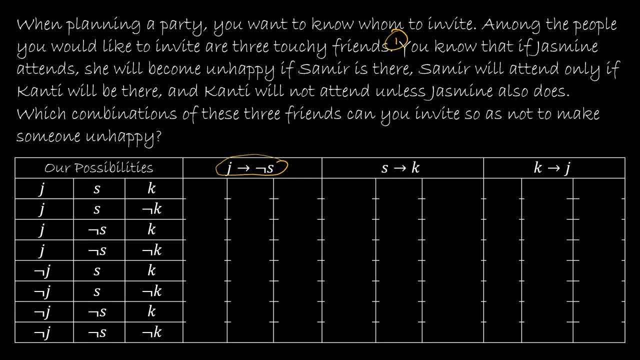 The second one was Samir will only attend if Chianti will be there. So I'm saying Samir implies that Chianti was there. I'm sorry, not Conti, not Chianti, which is alcohol. And then, of course, let's pick a different color. 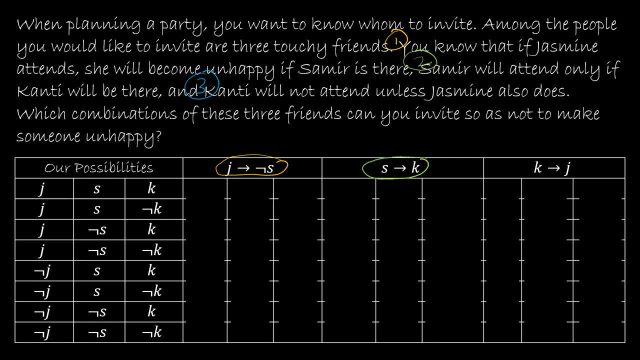 Blue, we say Conti will not attend unless Jasmine also does. So Conti implies that Jasmine was there. From here, the next thing I did was I took anything that was not on the implication side. So here I'm going to leave the S column alone. 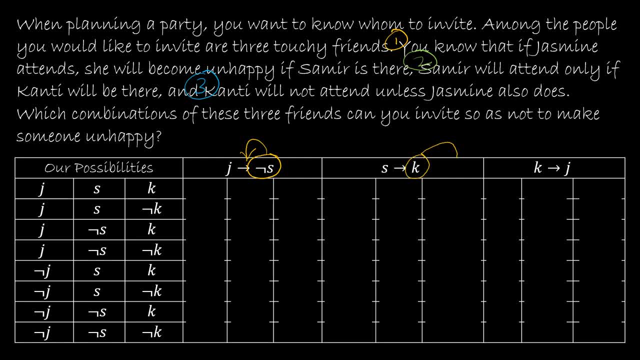 so that I can fill that in in a minute. I'm going to use the K column and fill that in in a minute, And I'm going to use the J column and fill that in in a minute And I'm just going to copy over everything else. 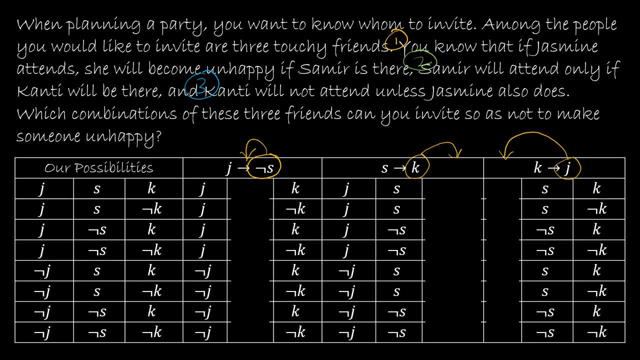 So notice the ones that I've put the arrows on. those are blank. So let's talk about where those solutions will come from. What I'm going to do is I'm going to take a look at the J value And if J is true, then I'm going to write, not S. 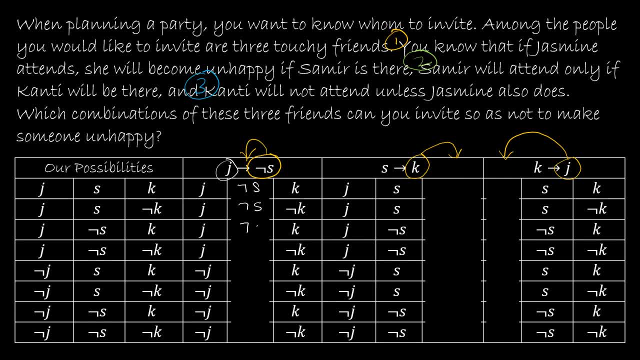 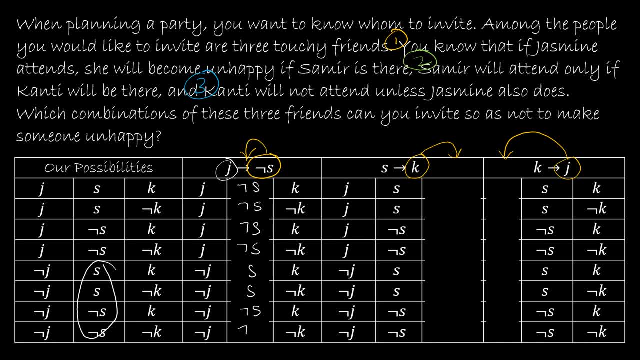 if that first part is false, then it doesn't say anything about the second part. So that's where I'm going to come up with those values. Now, from here I really can start to take things off of my possibilities. I need for everything in this row to be J S C. 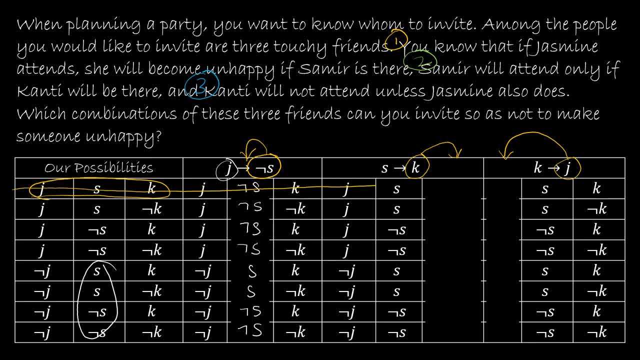 And already I don't have that here because I have J not S K, So I'm going to cross that off And I'm going to cross this one off as well, for the exact same reason. And J not S K. that one works out okay. 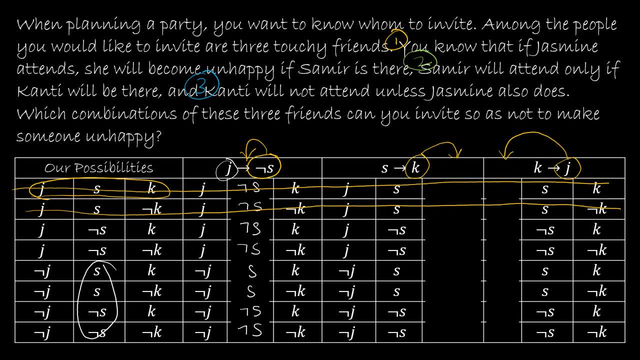 J, not S, not K. that one works out okay, Not J S, K is okay. That sixth row is okay, The seventh row is okay, The eighth row is okay. So so far I've done that. 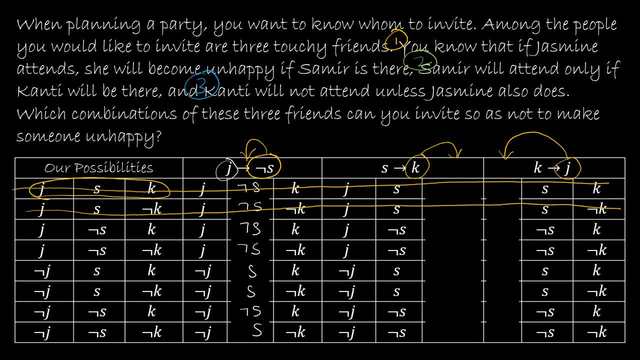 I've taken off everything in the first two, So I'm going to get rid of this, and just so that it's a little bit nicer writing. So again, we've crossed these off. Now let's take a look at the next one. 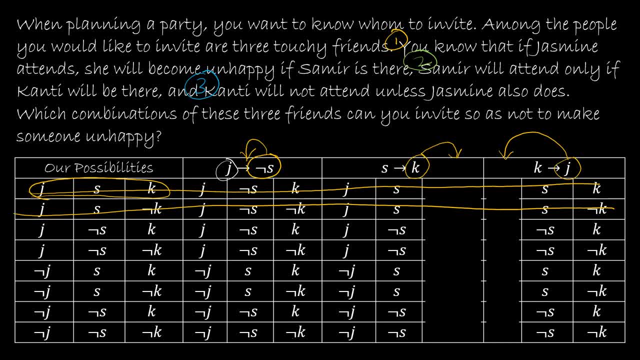 So S implies K. Again, that means if S is true, then K is going to be true. So I'm going to go ahead and fill in these And then, if not S is true, then we're just going to write whatever was here already in the Ks. 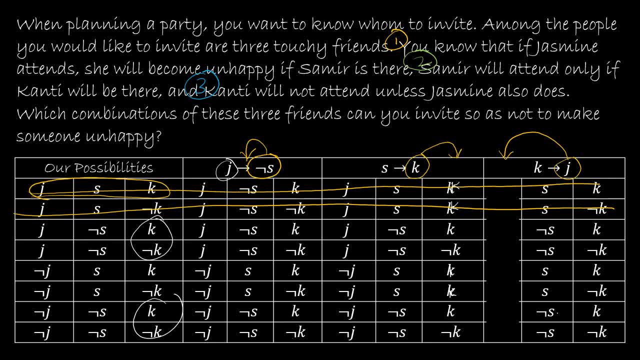 So again, I'm going to just uncover those to make it a little bit easier, And I think that's just going to keep happening. So I'm just going to keep this crossed off and this crossed off, And so now again I'm going to compare. 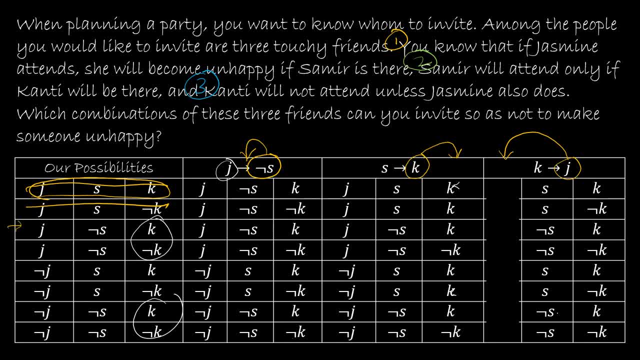 the original row: J not S K. And if I get something besides J not S K, then I'm going to cross it off. So J, not S K, that matches up. J not S, not K. that matches up. 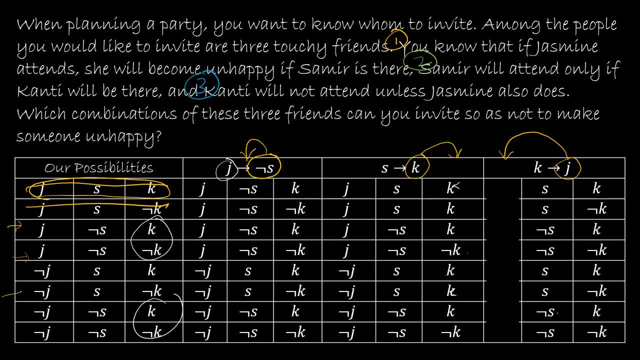 Not J S K. that matches. Not J S, not K does not match. So this one's gone. Not S, not J, not S K, that one's okay. And not J, not S, not K, that one's all right. 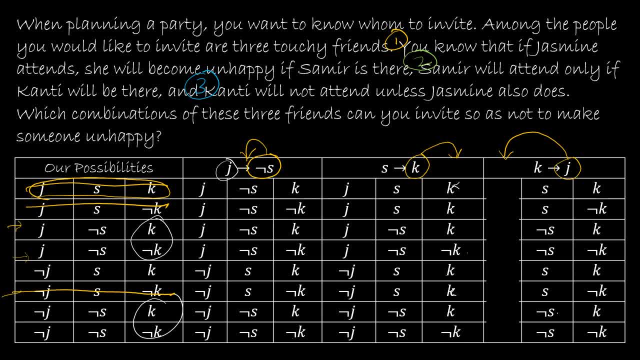 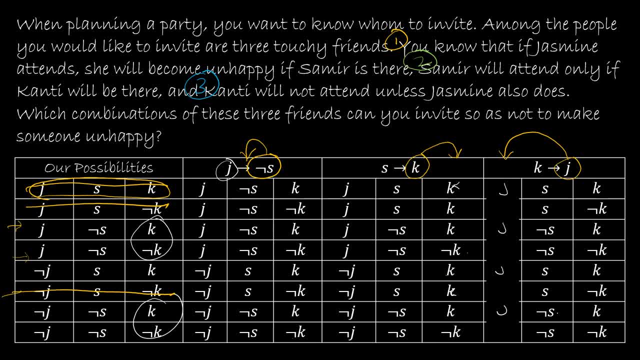 and the rest of them will be whatever happened in the original. So that would be J here, J here, not J, not J. And then again we're just going to compare. So we're going to compare J, not S K, and notice everything. 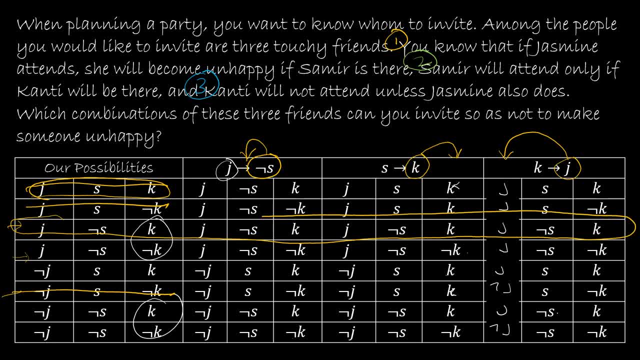 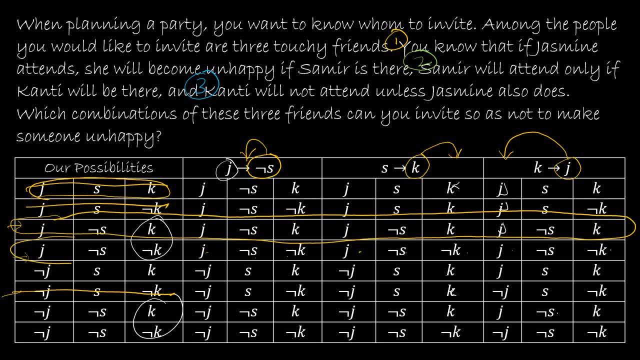 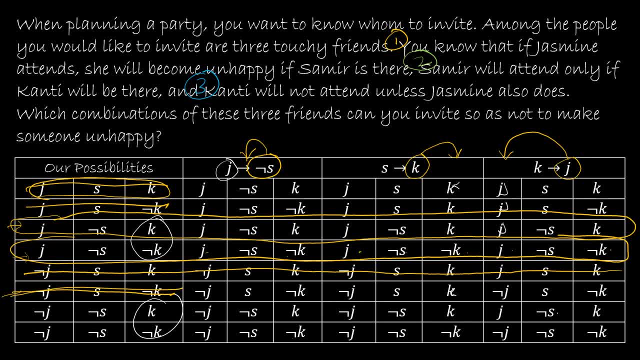 We already took off this one And we've got not J, not S K, And that one doesn't work because this one should be a, not J, So this one's gone. And then that very last row, I've got not everything, which is okay. 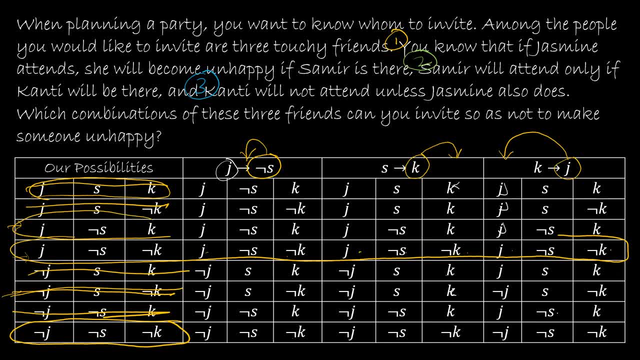 So here's what this boils down to. We had three where everything was the same all across the row, So let's just use a different color there to maybe highlight that. That would be here. Yes, please do make the sound effects with it. 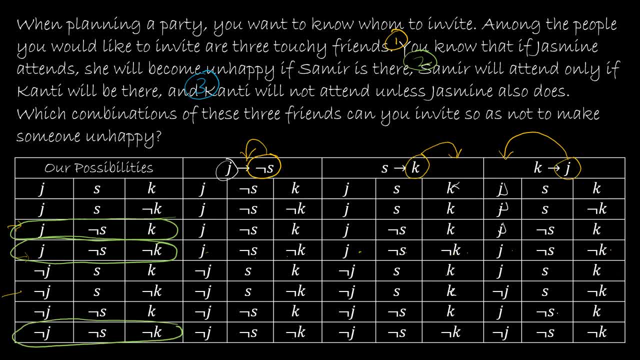 These were the ones that worked out for us. So what does that tell us? Who can we invite? We can invite J, not S K. That means invite Jasmine. don't invite Sameer, but invite Jasmine. We could invite Conti. 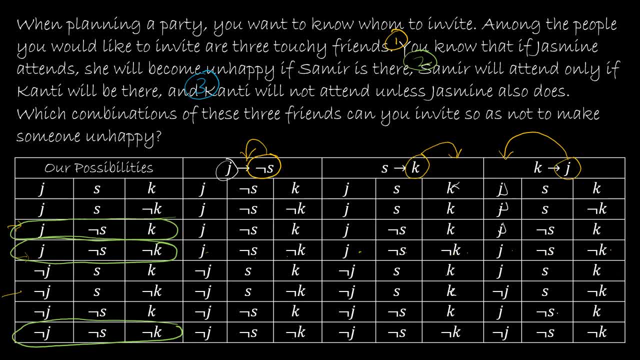 Or we can invite Jasmine and not, Sameer and not Conti, Or we can just say: y'all need to grow up and don't invite any of them. Those based on what we've given in the question, those are our possibilities. 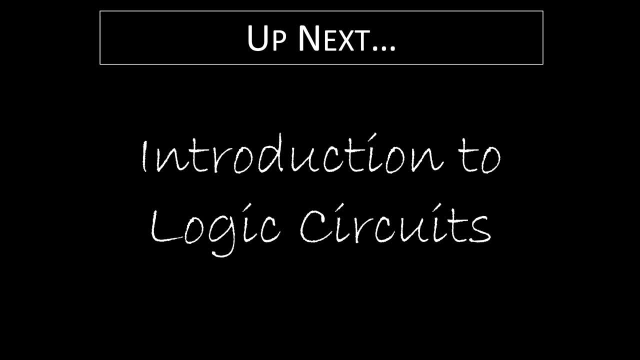 Up. next we're going to take a look at some logic circuits, which is basically a way to look at a propositional statement and to write it in a diagram.